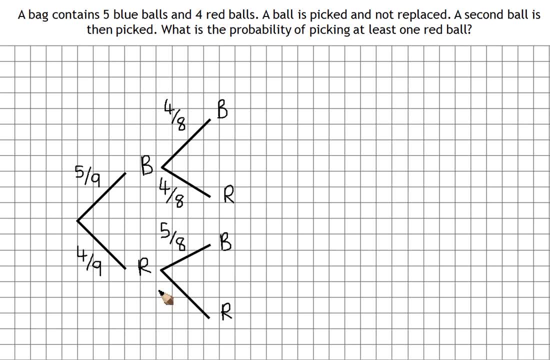 5. So we've still got 5 blues Along here, 8 balls left in the bag. We've already picked one red, so there'll only be 3 left. Ok, so you can see these probabilities along this branch, or these branches here are now different, To find the probability of picking at least. 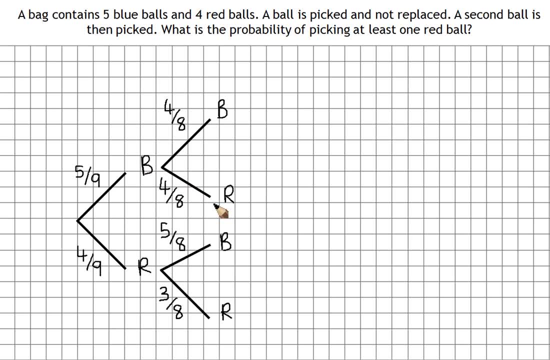 one red ball. the idea is still the same, though We've got this option. we've got this option and we've got this option. So if we want the probability of blue and red, we multiply the probabilities. So we've got 5 ninths times 4 eighths this time. So that's going to be 20 over 72.. For this branch, 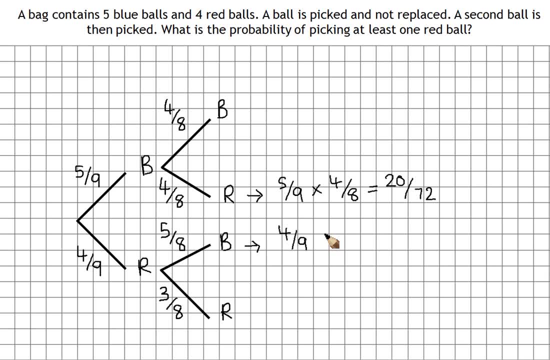 here we've got 4 ninths times 5 eighths, So again 20 over 72.. So that's going to be 20 over 72.. And for this branch here we've got 4 ninths times 3 eighths, Which is 12. 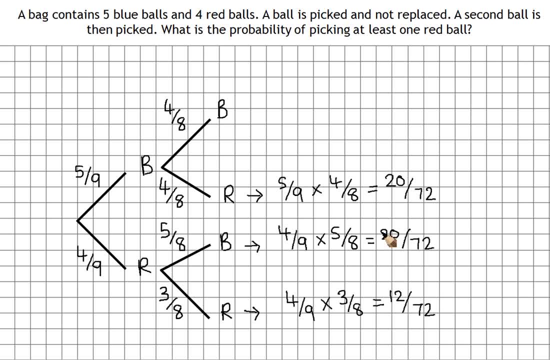 over 72. Now we want this one or this one or this one. So my final stage is then to add those probabilities up, So 20 over 72 plus 7 over 72. So we've got 20 over 72 plus. 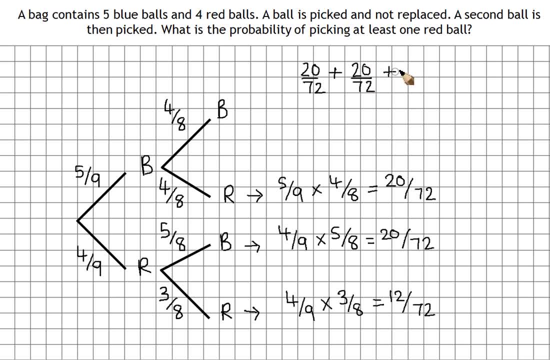 20 over 72, plus 12 over 72, gives me 52 over 72. Now, if the question asks for it in its simplest form, you need to cancel this down. So you should realise that both of those can be halved.